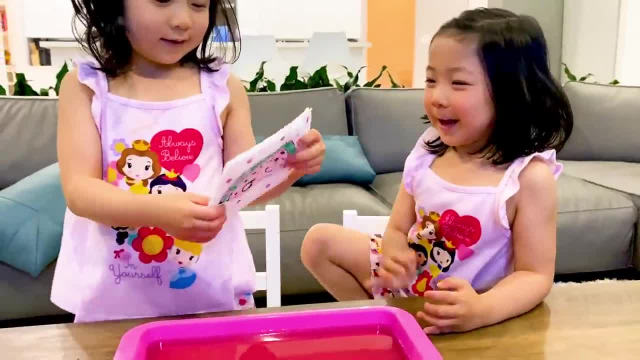 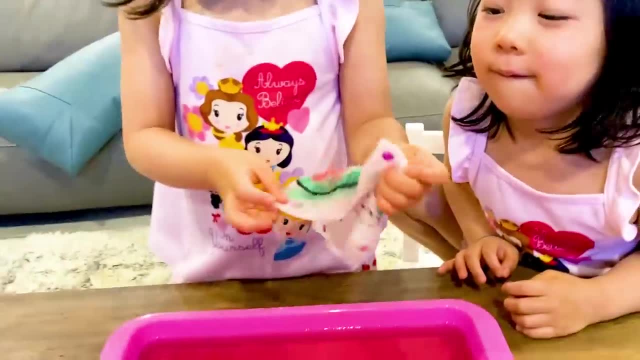 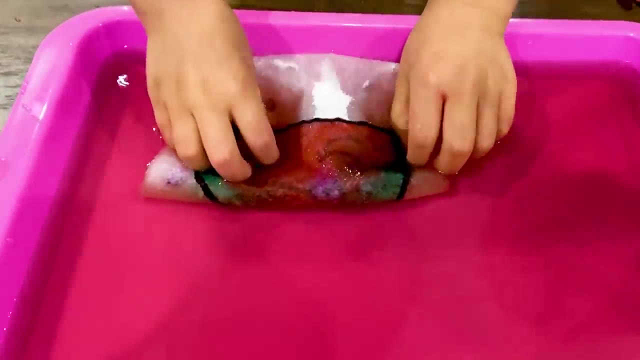 I think it's water. Really, I think it's a rock, A rock, Let's see. It's greener, right, Yeah, And red, So it's just- almost correct. Let's see the rest. Wow, I'll show you what it is. 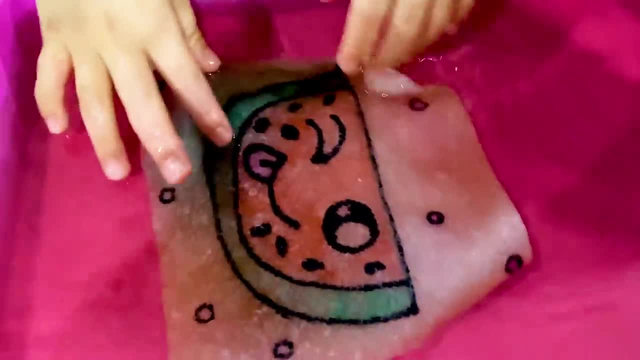 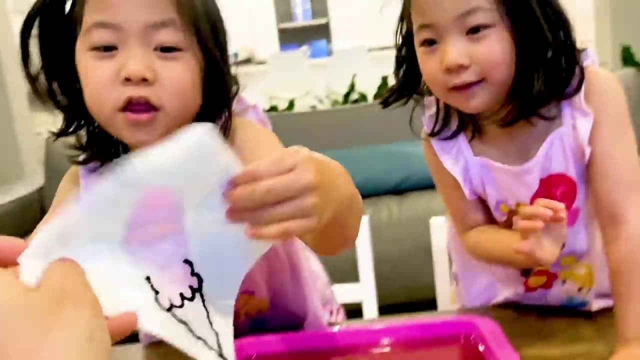 Aw, it's a cute watermelon. There it is. Now I choose, You choose one, Okay. So what is this? Look, it's like a triangle and we don't know what it is. I think it's the ice-cream. I mean, I think it's a rock. Well, I think it's the ice-cream. 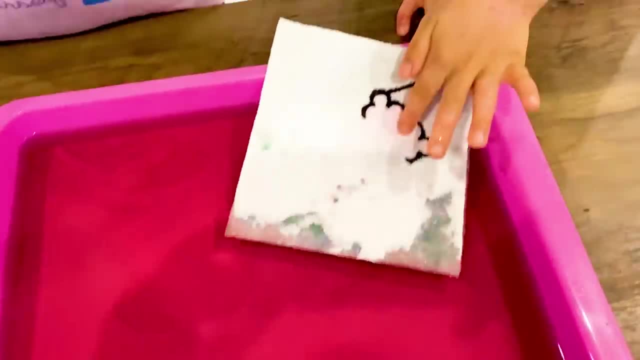 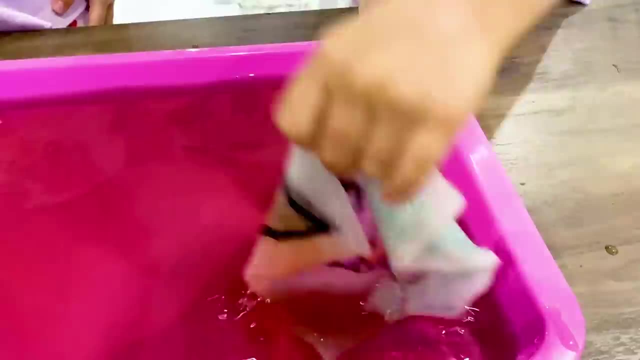 Okay, let's put it in and see, But a lot of water. Yeah, now I'm putting these in. Oh, It's a lot of ice cream. Okay, Wow, Whoa, Kate's right. Yeah, look guys, it's a lot of little ice cream. 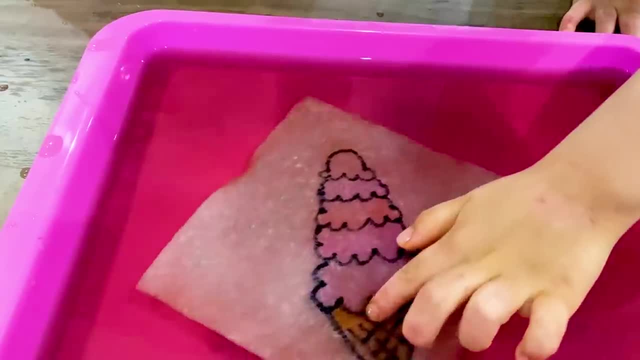 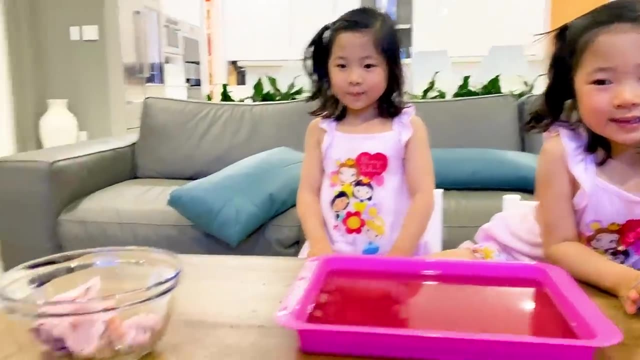 Oh, yeah, you're right, Kate. How many? How many scoops? Wait one, two, three, four, five, Five scoops of ice cream, that's a lot, huh, Okay, it's Emma's turn and look, all she has is heart. 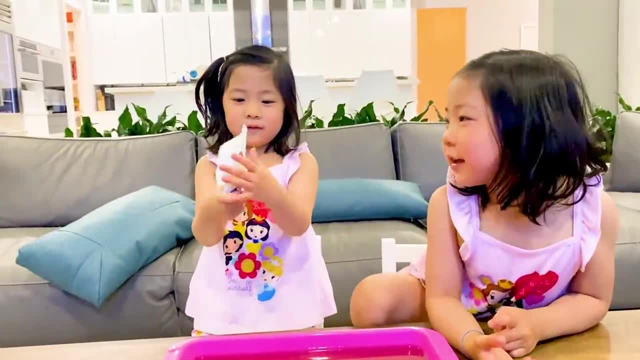 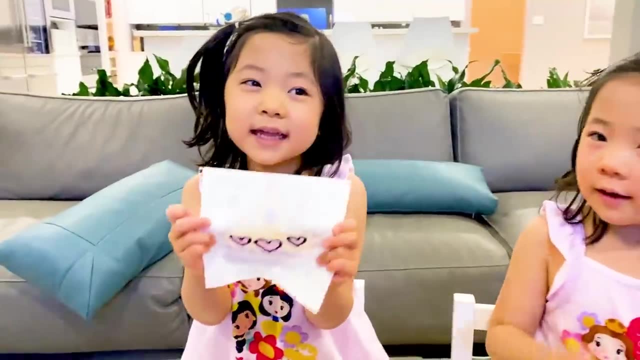 Let's see what happens. I think it's a rock. A rock. I think it's a crown, I know. Okay, what about you? I think it's a real crown. Okay, let's put it in, Let's see. let's see. 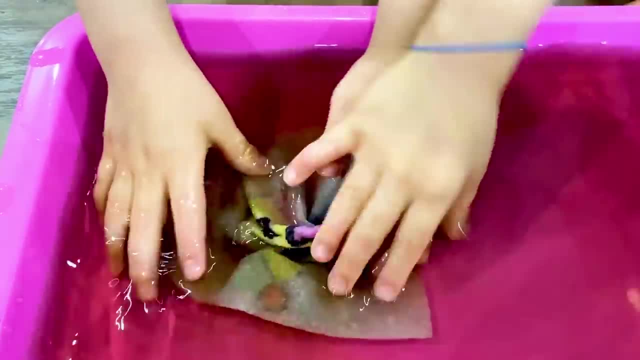 Whoa, what is it? I want to put it on top. Can I put it in my hand too? Yeah, it's a crown. Did you guys see a crown? I can't even put it there. Okay, Kate's turn and look. 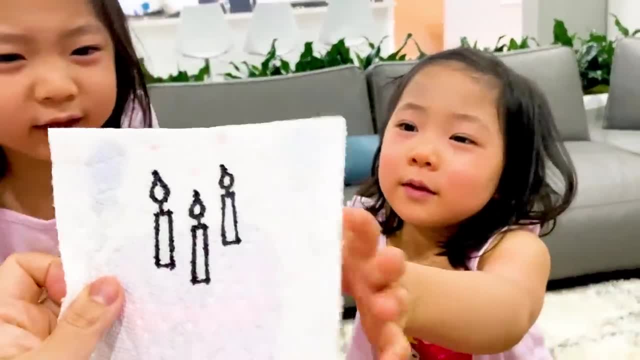 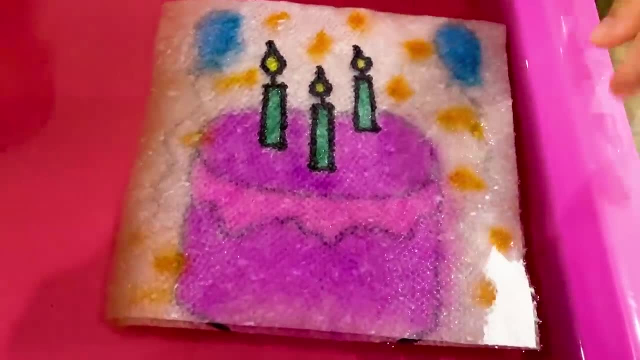 all we have is: how many candles do you see? I only see three, Three. I think it's a cake, A cake. I think it's a rock cake, A real, real cake. Yeah, That's correct, I'm gonna show you. 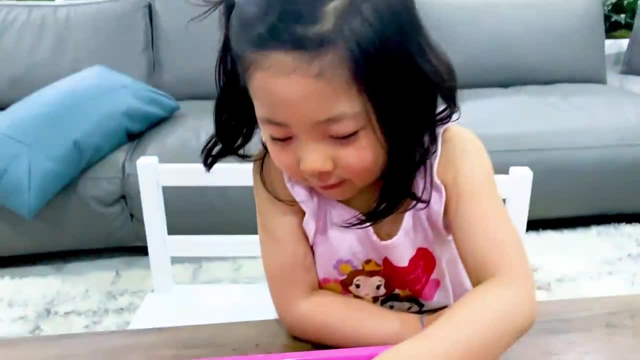 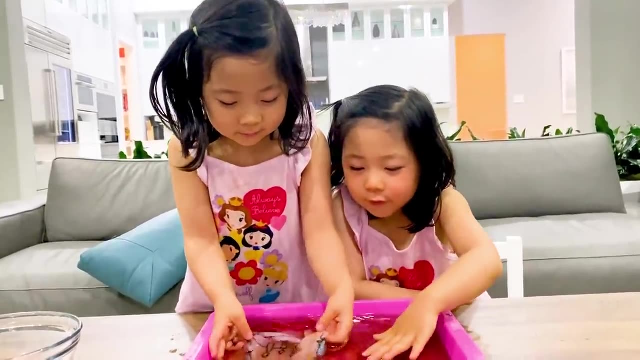 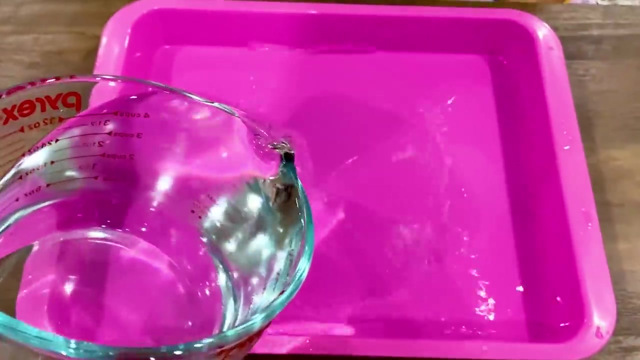 Yeah, Happy birthday to you. It's like Emma Kate's birthday. Happy birthday to you. Happy birthday to Emma Kate. Happy birthday to you. My hands are dark. Your hands? Yeah, Hey, fresh, clean water, Wow, Okay. so what is this? 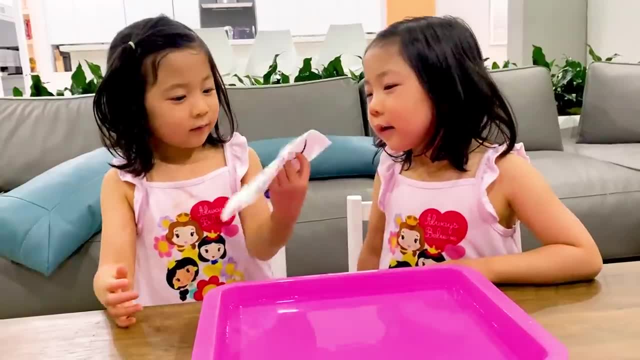 A bunny museum. I think it's a Bum, bup, bup, bup, bup, bup, bup, bup, bap, bap, bap, Bop, bop, bop, bop. 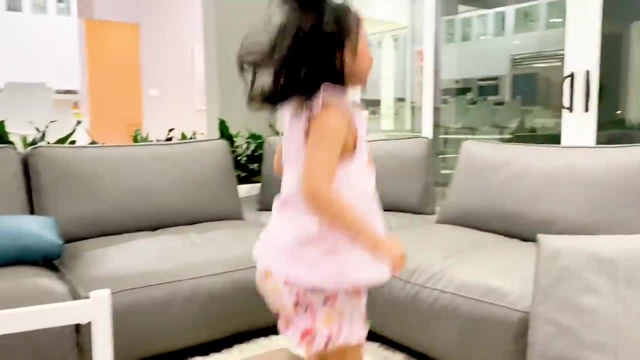 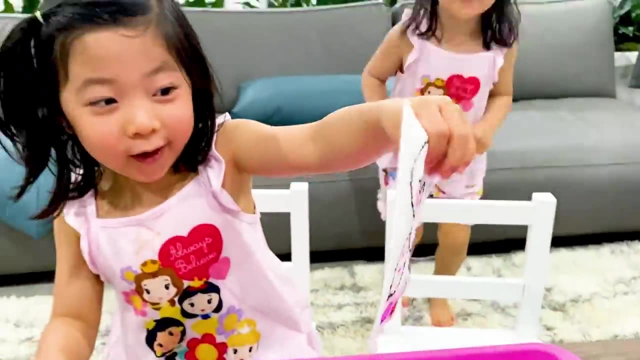 Hoppy A hoppy, Yeah, like this. Hoppy, hoppy, hoppy. Like this. Let's see Hoppy hop, bop. Like this: It's big right. They're right. I must come back to Emscraft. 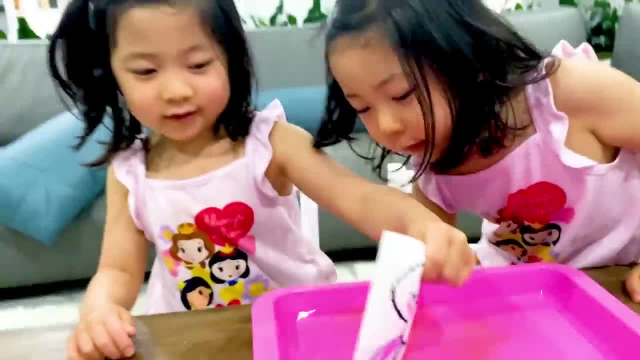 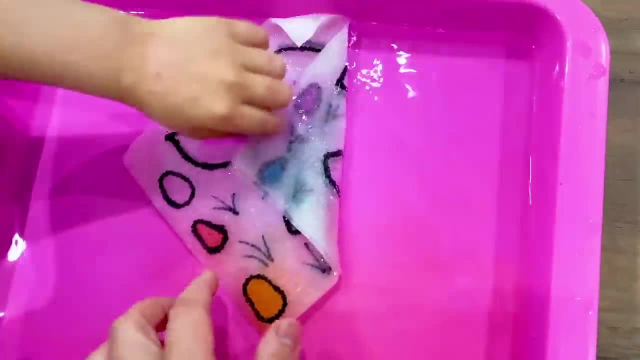 She's doing it like: Wait, the color's not enough. The color kind of got off. See Emscraft: Whoa, that's beautiful. Look on the other side, it's super beautiful. huh, Yeah, But now the water's turned pink. 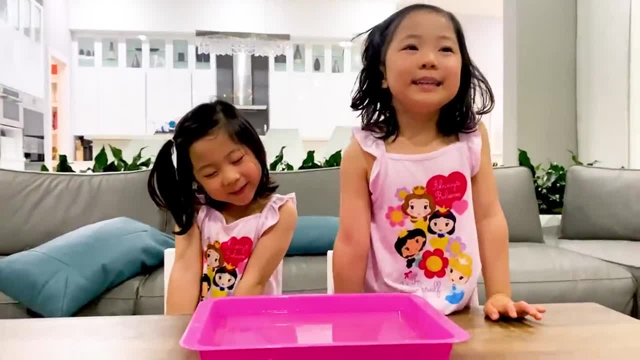 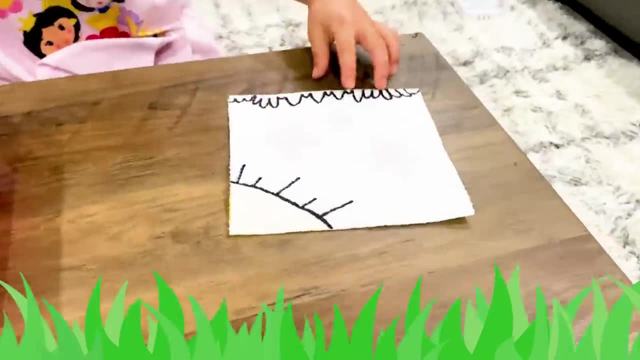 It is. How do you lift it up? The color's coming out. You guys see it. Okay, Kate's turn. All you see is a sun. Let's see what happened when you put in water. I think it's a beautiful garden. 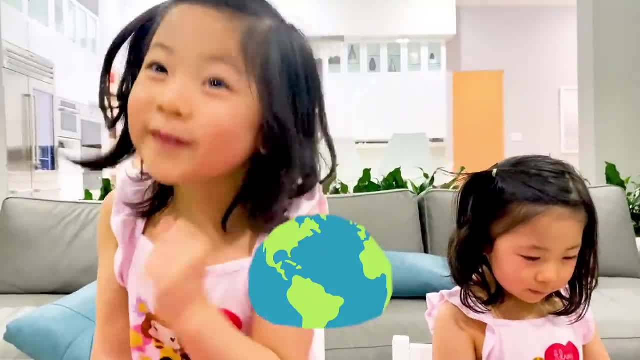 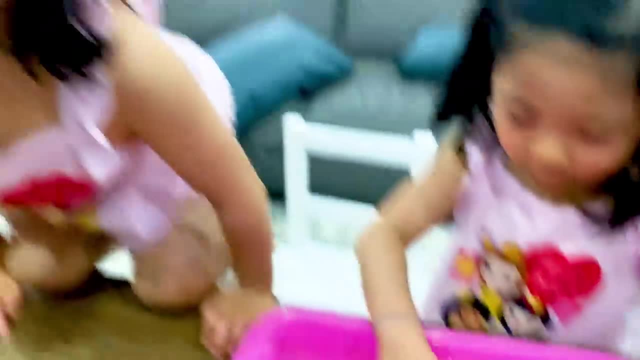 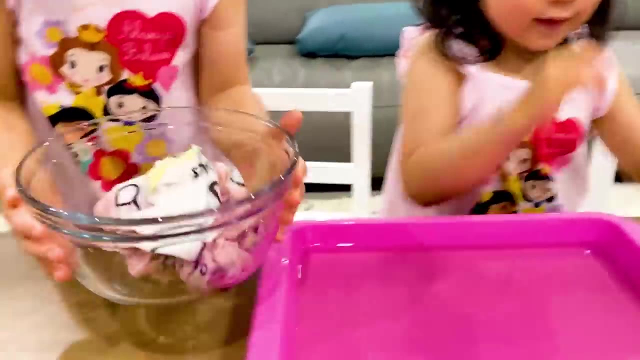 You think so, And I think it's a rock world. Kate's right. Kate, you're right, It's a beautiful garden with flowers. Hi, Mommy, Hi, I love you, Kate. Good job, Kate. Okay, now Emma's turn. 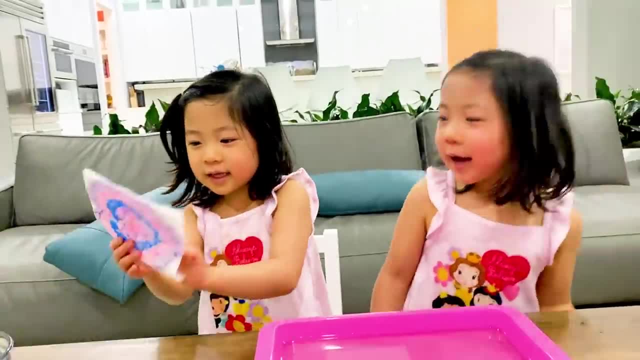 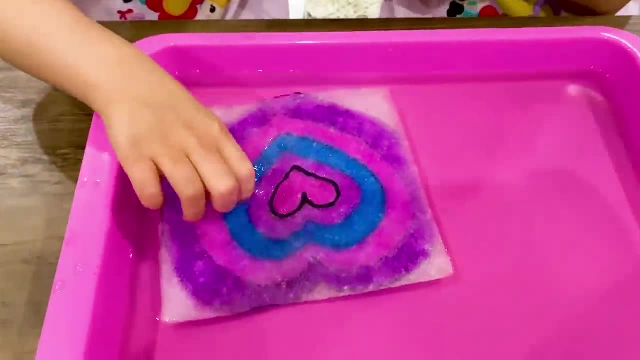 All you see is a baby little heart. Let's see what happened when you put it in water. I think it's a love heart, A love heart. I think it's so much fun. Okay, Me too. That's what I mean. 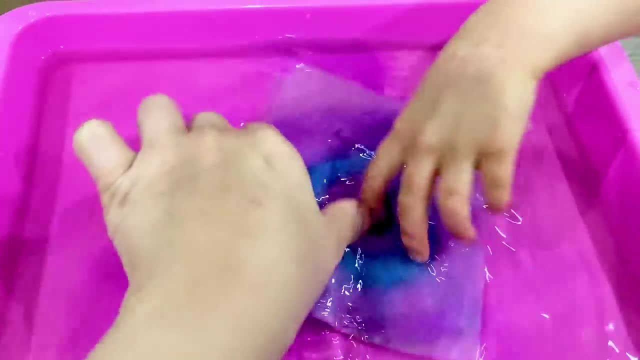 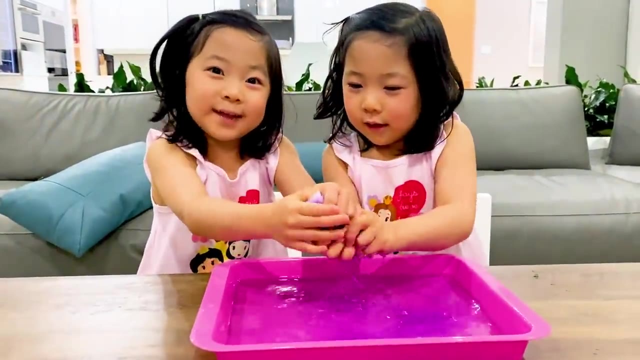 That's what you mean, Like a big giant heart, like this, of love. That's fun. It's fun, Spin it, Spin it. Let's say: twist the bag, Twist, twist, twist. Okay, guys, Now that you guys have done it, was it fun? 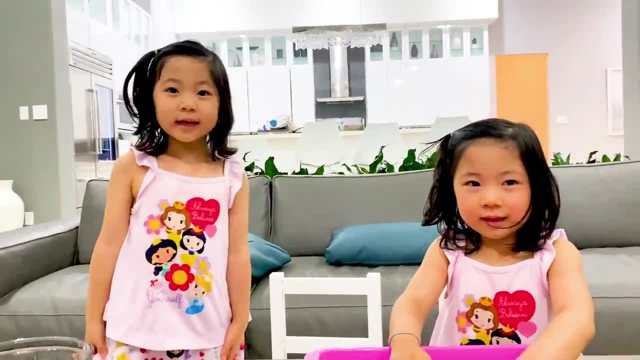 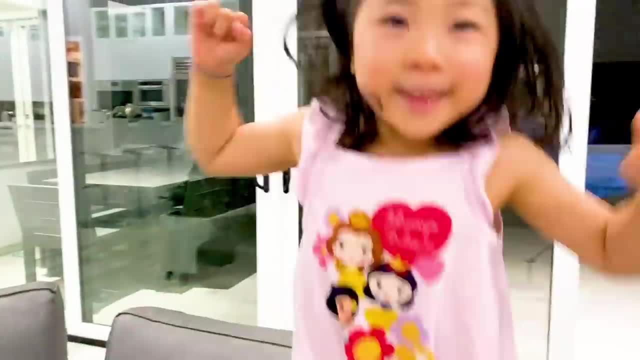 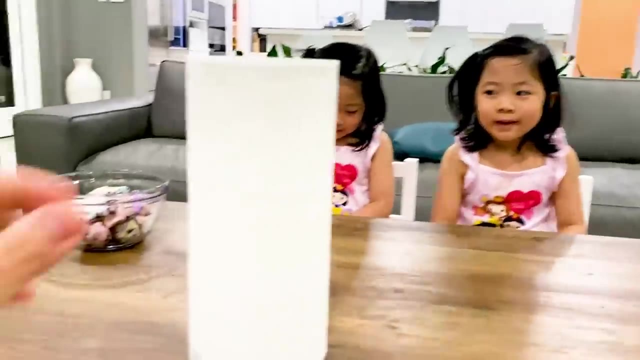 Yes, You guys want to make your own? Yeah, Yeah, Okay, I'll be right back. Are you guys ready? Yeah, Yeah, Yeah, Jump, jump Up and down, Up and down, Hi, Hi, Okay. so all you need is a paper towel. 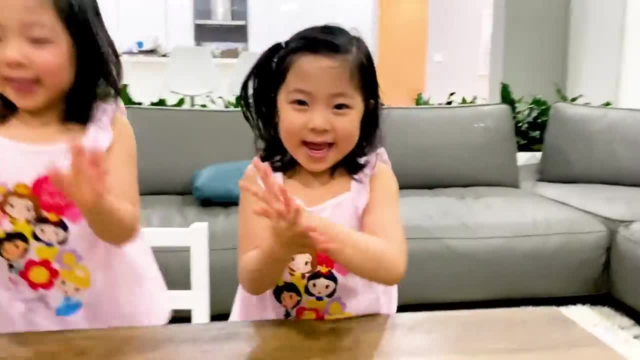 I'm going to give each of you And a color marker. That's right, Color marker. Okay. one for you, Thank you, And then one for you, Thank you. I'm going to draw two while you guys do it, okay. 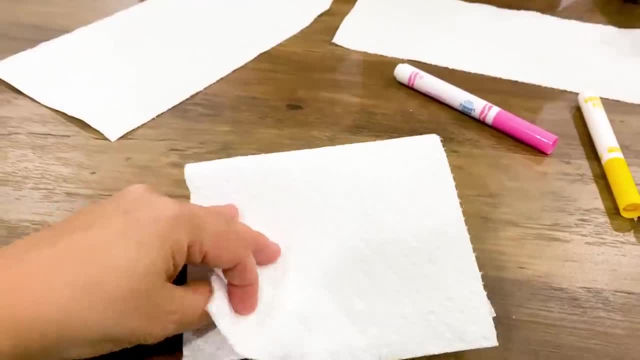 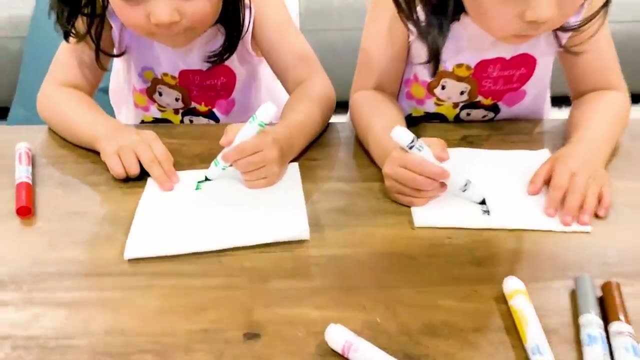 So all you need is a sheet of paper. then you fold it in half A little more. Yep, Okay, for you too. Now we're going to make a black. Fold it in half like this. I did it, Yeah, so draw anything you want. 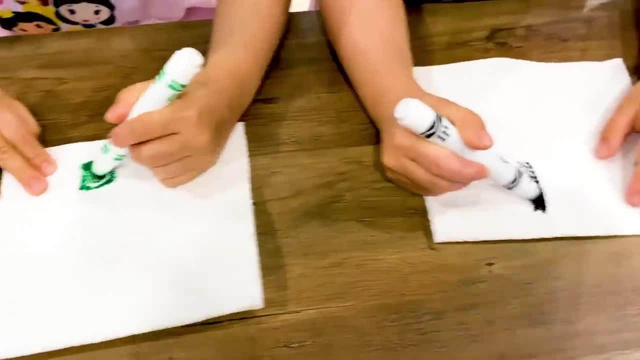 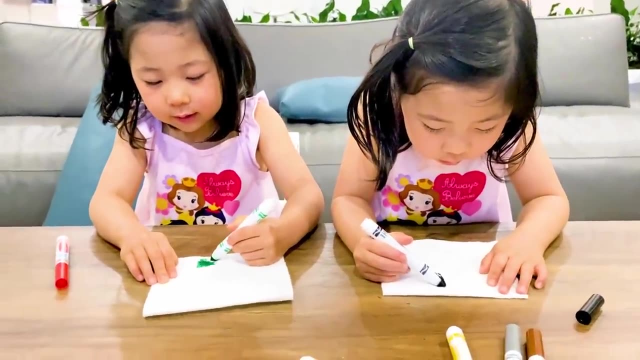 I'm going to draw Munchy with a baby. Okay, No, it's too much. Perfect, She had a green. I know she's black and mean She had a green tail. like this: She has a green tail. That's her green tail. 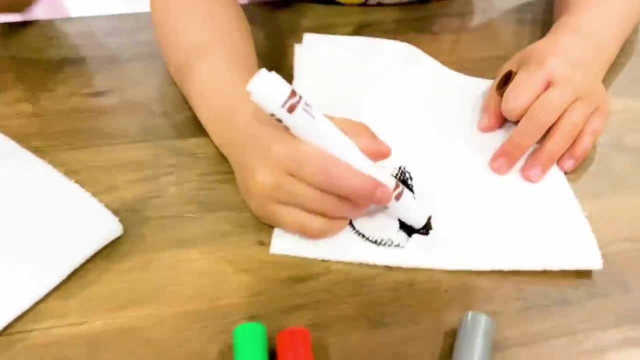 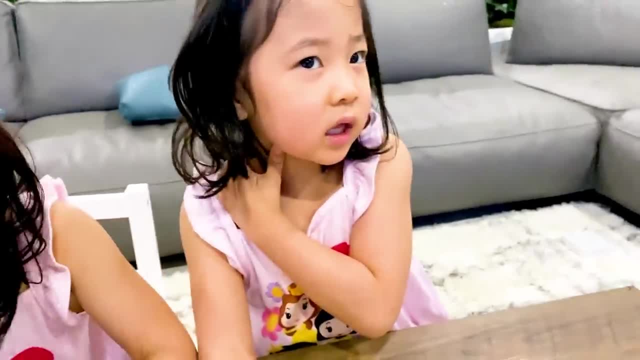 Because I don't remember how she looks like. You think she has brown hair, Ursula, I don't remember either. Okay, so Emma drew the face. You guys see the face here, Look. Oh, that's cool, I like it Emma. 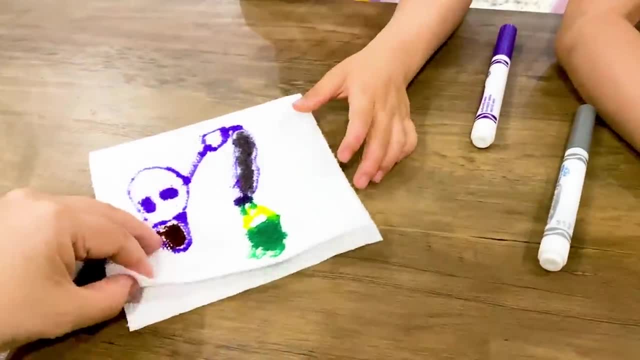 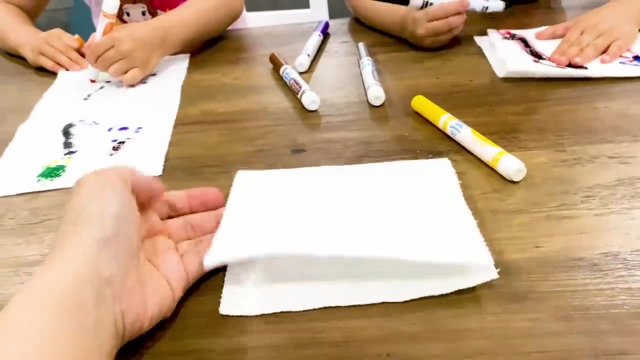 And her dress Okay. so when you're done with the front there, then you just flip to the back side and draw something here too- No, it's too much, Because you got to save size. It might turn too, And if you don't want it to leak, you can just do one like this: 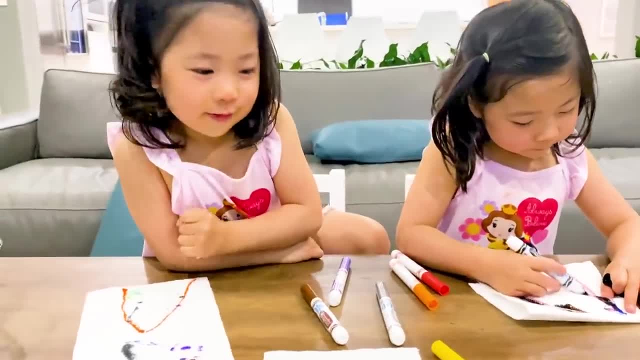 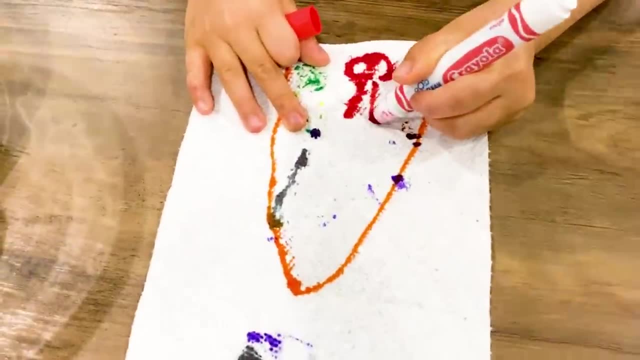 I'm going to draw a majesty stuck inside. Oh, that's a good idea. There You're done, Okay, and then you flip to this side and you draw something here too. Okay, Emma, Okay. so on this side, that's what Kate is drawing. 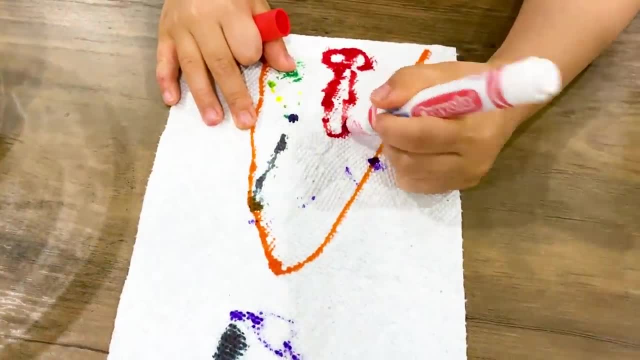 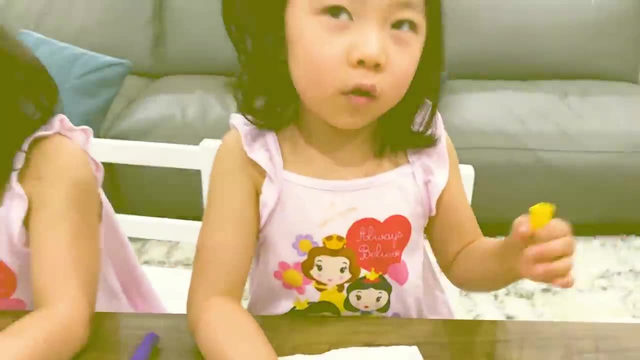 That's cool. What is it? A mountain, A cage? Good, Emma's drawing something too. That's cool. Emma, She's all yucky when she's on Superpower. I think I'm going to draw somebody with Superpower. 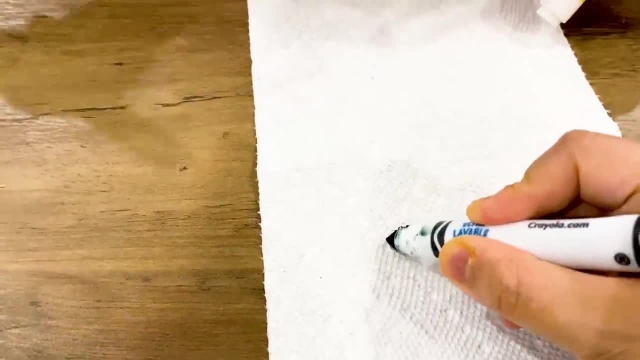 That's a good idea. I think I'm going to draw a face. Okay, that one, When you draw You can use, like: that means bungler. You want to make a bungler? Okay, yeah, bungler. 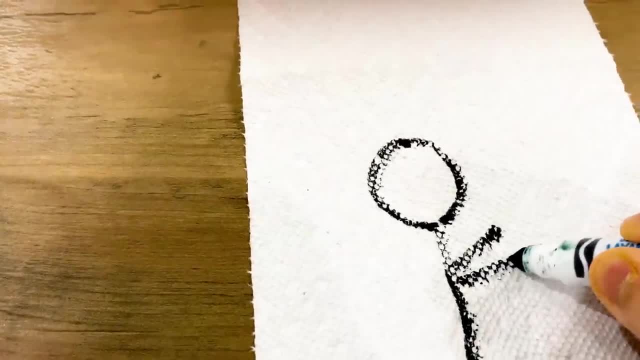 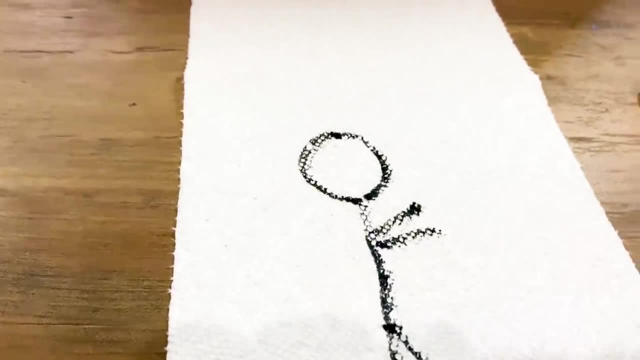 And then it has little arms. Now I'm going to do another one. I forgot about arms, You forgot about arms, It's okay. And then here's the leg: Okay, and it's a Superpower girl. so you'll see. 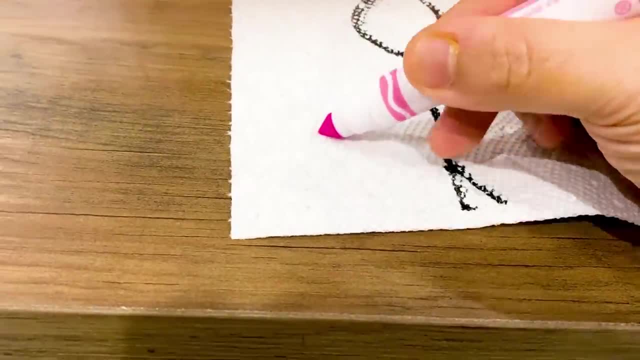 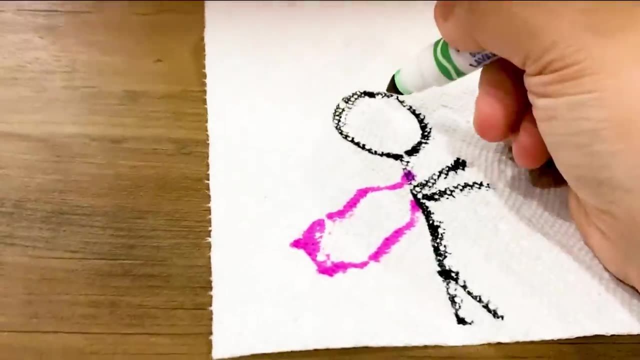 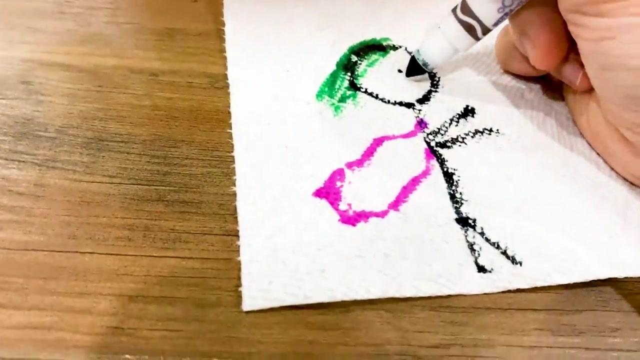 You got to use black. And then I'm going to use a cape because she's flying in the sky, Okay. And then I want my Superpower girl to have Green hair, So that's kind of cool, Okay. and then here she's smiling. 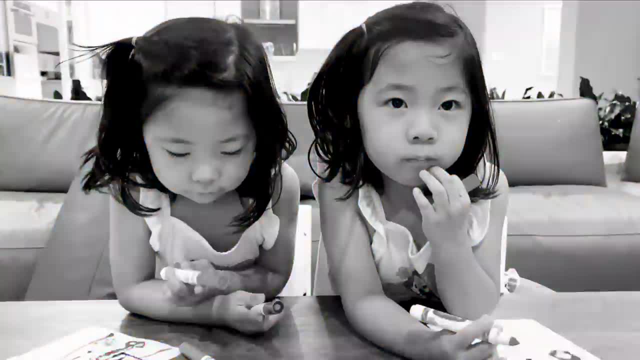 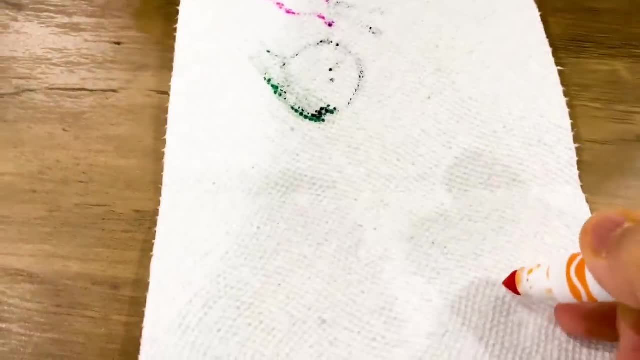 See. So basically I'm going to draw the evil person. on the other side, I'm drawing the evil person too, Really Okay. So on this side here I'm going to draw like an evil monster, maybe, But you don't know how to make an evil monster. 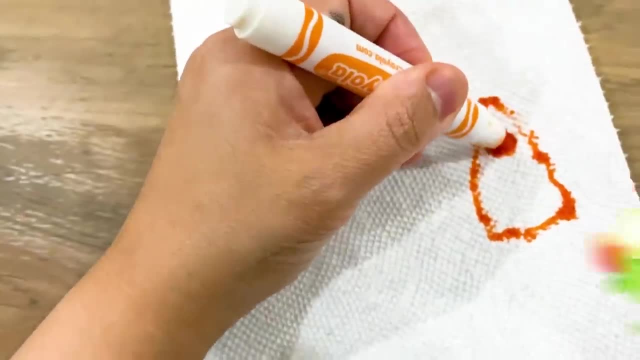 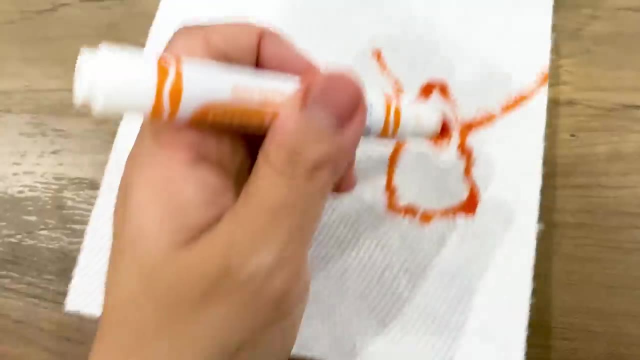 But the evil one? I don't know either. Maybe this is my one-eyed monster. I'm going to draw a monster. I'm going to draw a monster. See a monster, You guys see a monster? Yeah, Okay, It looks like. 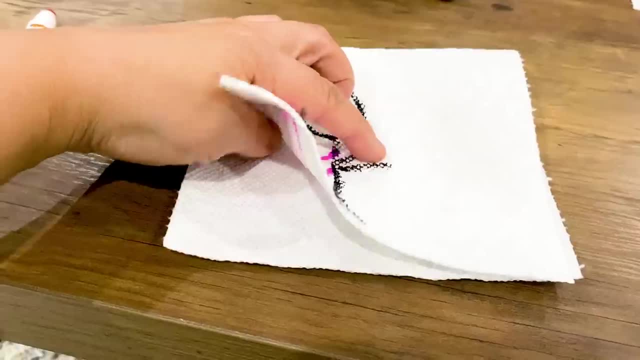 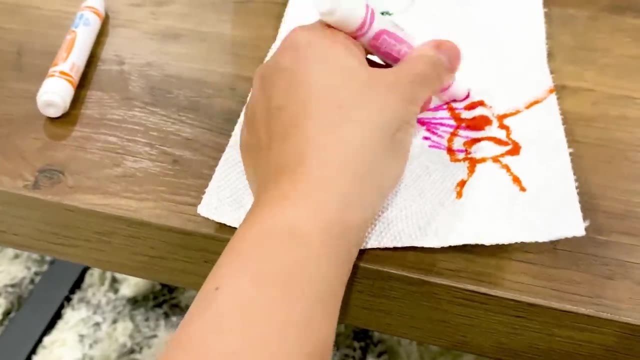 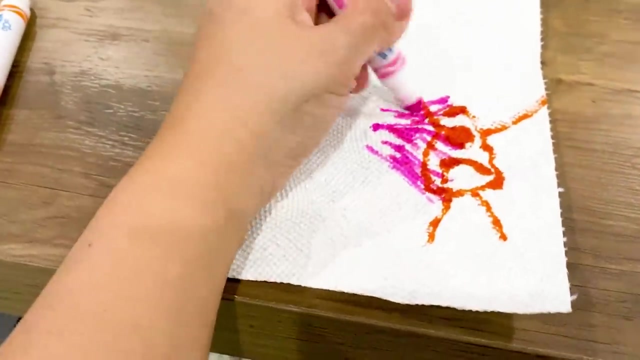 A sad monster- Sad, Not a happy monster. So I want the power to blast out from her right here Like lots of power at the monster. But you don't see that yet until you put it in water. You don't see this until you get in water. 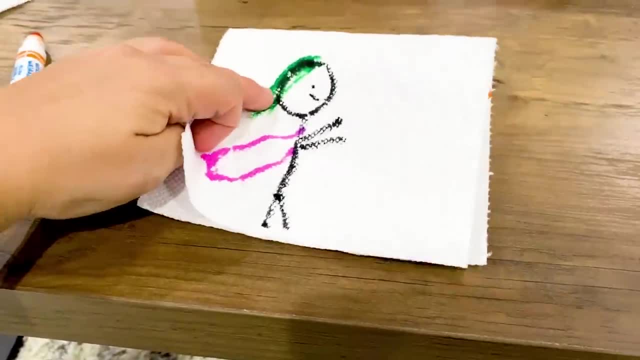 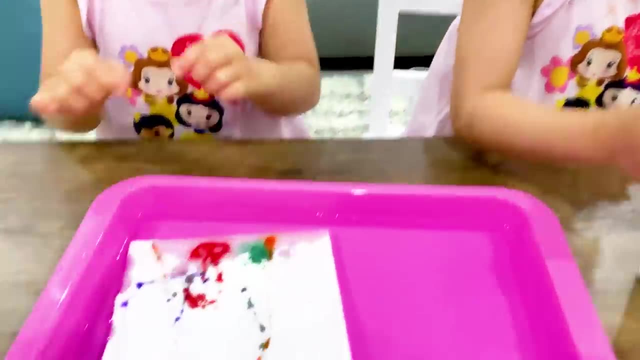 Okay, there, it is All right. Okay, All right. So when you're done with your drawing, just put it in water. So here's Kate. Kate goes first. Let's see what it looks like. Whoa, You guys see. 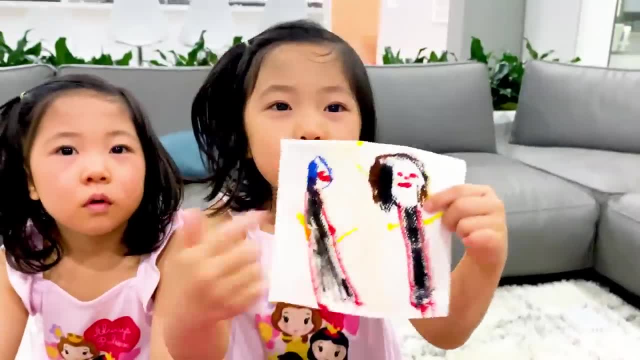 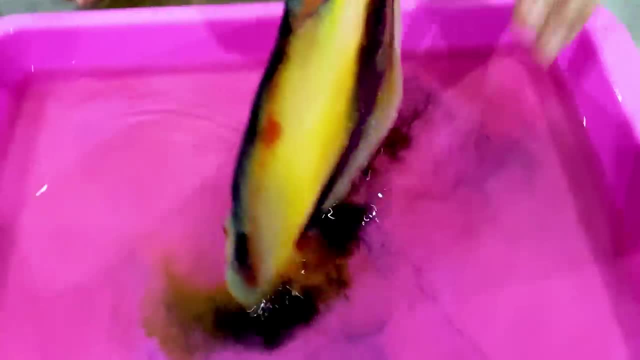 That looks really cool. Okay, So that's Emma's drawing. That's Emma's turn. That's right. Whoa, Do you see the yellow that came out from the back? Good job, Oh, look at the color that came out. 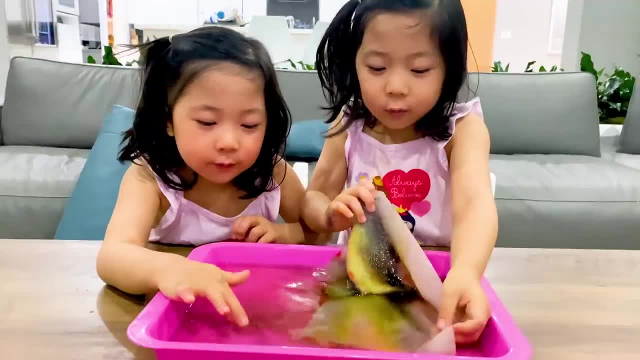 Look at that. Yeah, Let me see mine too. I know it's dark because I made the hand. Let's see if mine works, Okay. So look at this picture. It just looks like one person, right, He's doing that. 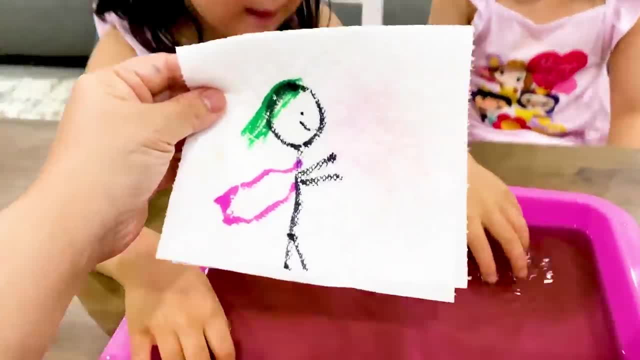 Yeah, He's by himself. So here you don't see the monster, but let's see what happened when you put it in. Let's see, There it is. See Shooting laser power at that monster. Boom, boom, boom, boom boom. 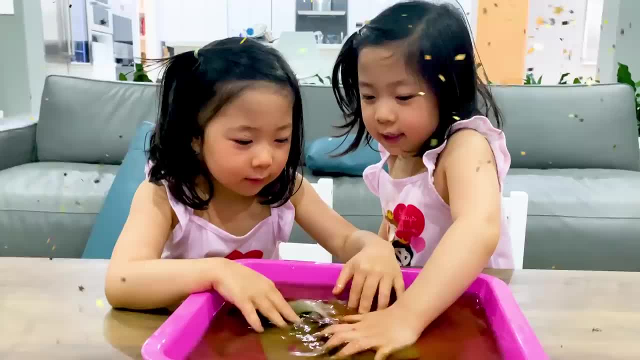 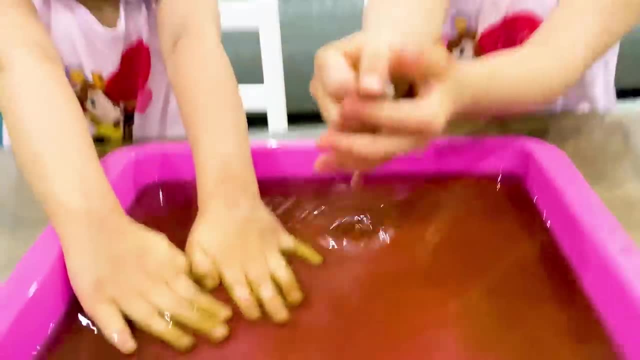 Am I correct? Yeah, Kate, You're correct. Good job. So there it is, guys. That's how you do your own fun water trick with paper towel. We're just throwing you. Yeah, Look, Bye, Bye, See you next time. 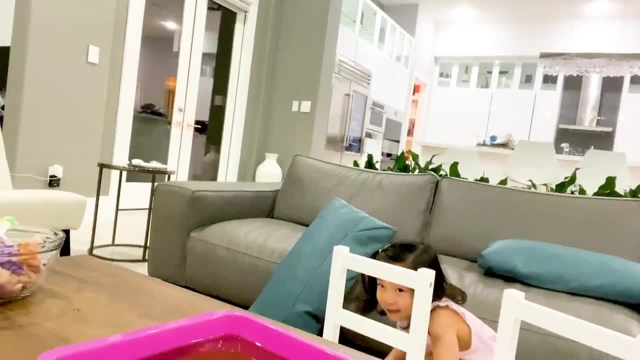 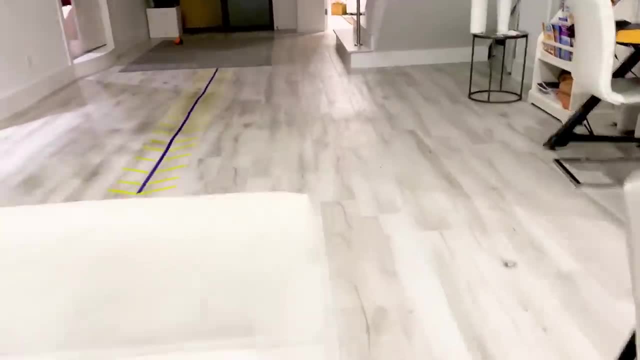 Bye, Bye. They love to hide. Where are they? Where are they? Where are they? Oh, where could they go? Where could they possibly go? Pokey, Pokey, Bye, Bye. Where's the other one go? 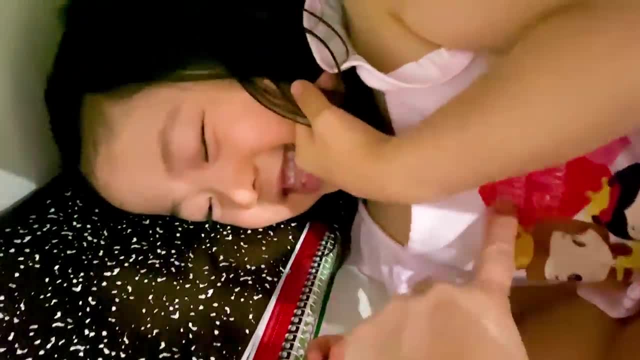 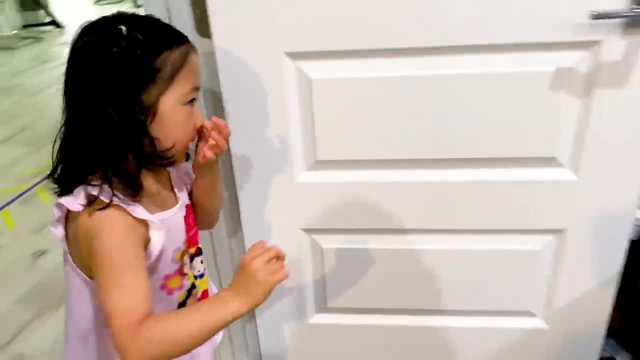 I think she went the right way. Where? Where Is she in there? I don't know. Yum, She just went the right way. Is she in there? Yes, Okay, Okay. So they're both in there, Yeah. 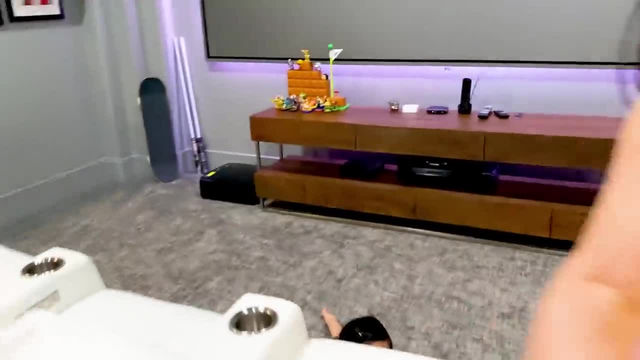 No, Hmm, Ashley's a good hider. Found her. Oh, There you are, Bye, Bye.